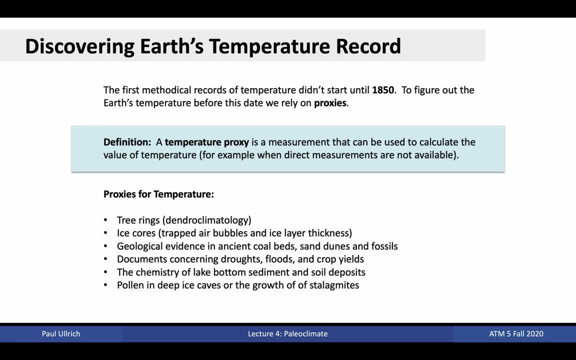 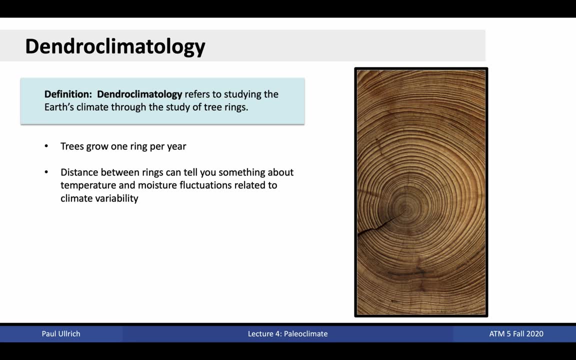 soil deposits or pollen in deep ice caves. At UC Davis, there are even researchers working on using stalagmites in caves as proxies for precipitation and temperature. in California, Over the past thousand years, we have obtained accurate measurements of temperatures by looking at tree rings from both cut and fossilized trees. Using tree rings as a proxy for climate is so. 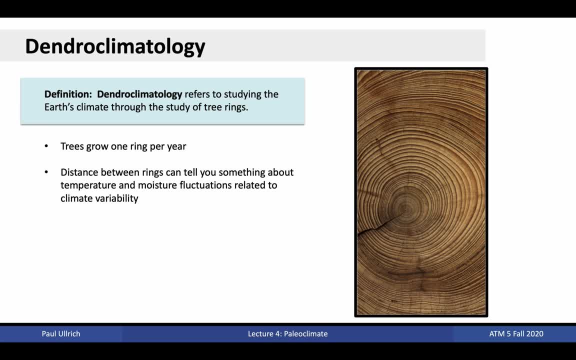 common that there is even a term for it, namely dendroclimatology. The basic process is simple. We know that trees grow one ring per year. If we measure the distance between adjacent rings, then it can tell us something about temperature and moisture fluctuations during that period. 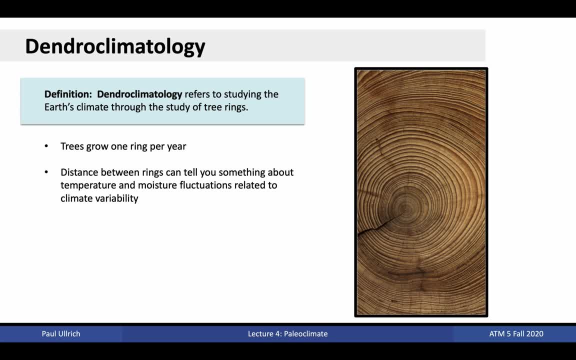 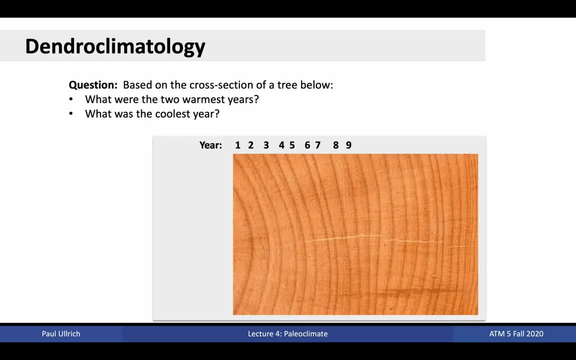 If conditions are warm and favorable for growth, then the ring will be thick. If conditions were cool, dry or otherwise unfavorable, then the ring will be thin. Look at the tree cross section below. Nine growth years are included on this figure. Which do you think were the two warmest years? Which do you think? 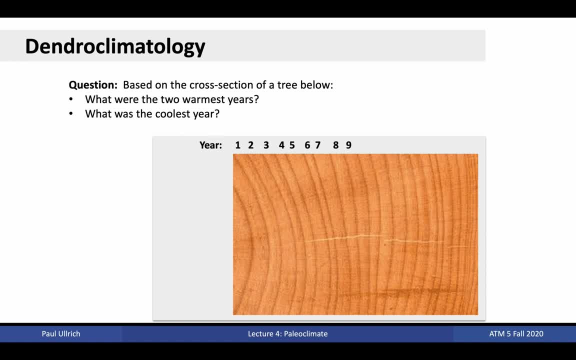 was the coolest year, Yeah, so years five and seven both showed significant growth, so they are probably warm years favorable to that growth. Year six, on the other hand, seems pretty unfavorable, probably because of cold weather, and the tree ring only grew a bit. 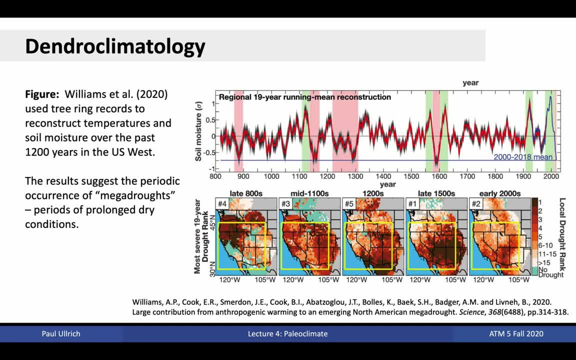 A paper by Williams et al in 2020 actually used these tree ring records to reconstruct temperatures and soil moisture over the past 1,200 years in the US West. The results suggested the occurrence of periodic megadroughts: droughts of significant severity that lasted. 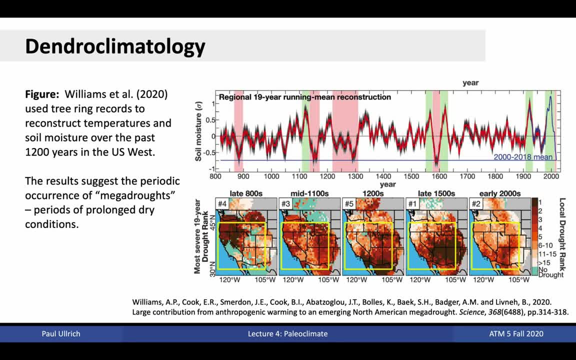 for decades to over a century. One such megadrought is implicated as a possible driver in the collapse of indigenous of the indigenous and Anastasia civilization in the US Southwest in the 13th century. Modern civilization in the US West has actually existed in a relatively 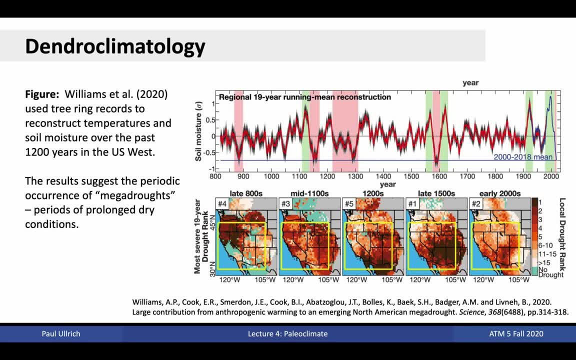 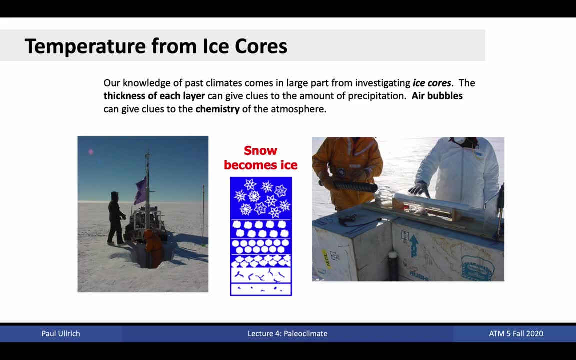 wet period conducive to agricultural production. However, there is evidence that we are now descending into another potential mega-drought event kicked off by human activity. Tree rings are excellent proxies for the past 1,000 years and have even be used to successfully. 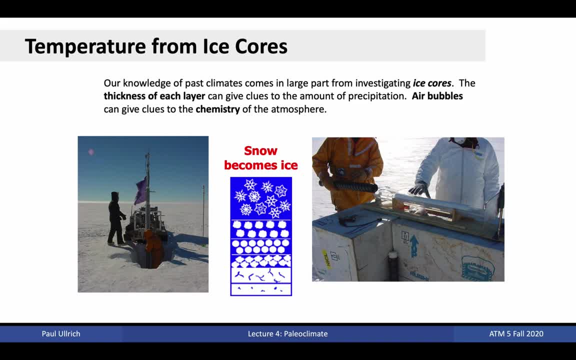 reconstruct. source: END OF TRANSCRIPT: a record of solar activity for the past 11,000 years. However, ice cores can be used to go back even farther in time. Much like tree rings, ice cores are stratified into layers, The thickness 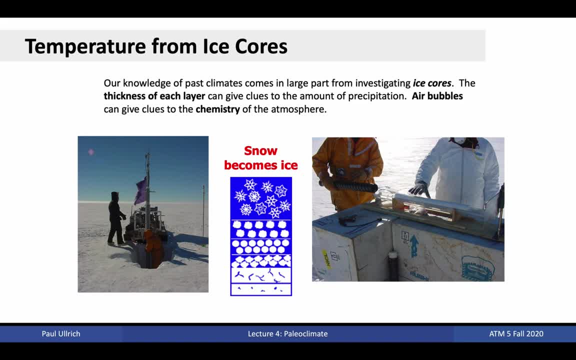 of each layer can give clues about the amount of precipitation that has occurred in that year. Further, air bubbles trapped in the ice can give us a snapshot into the composition of the atmosphere when that layer was formed. Ice cores are available from a surprisingly large number. 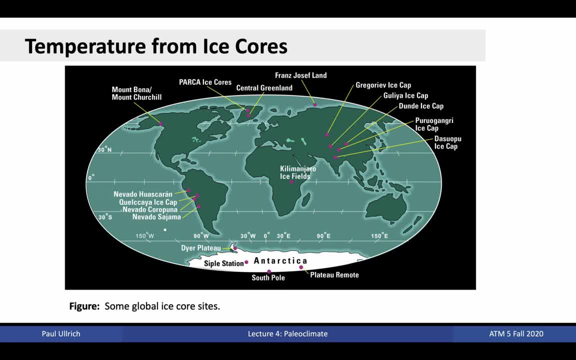 of sites worldwide, spanning most latitudes, Even right at the equator, the Kilimanjaro. ice fields atop Mount Kilimanjaro have provided a 12,000-year climate record in Africa. Other ice cores have come from glaciers around the world, including the Andes, the Alps, Alaska, the Himalayas. 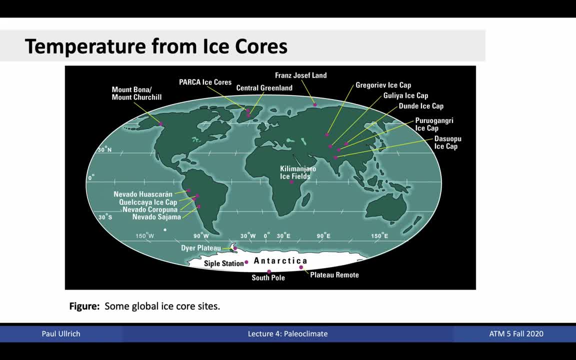 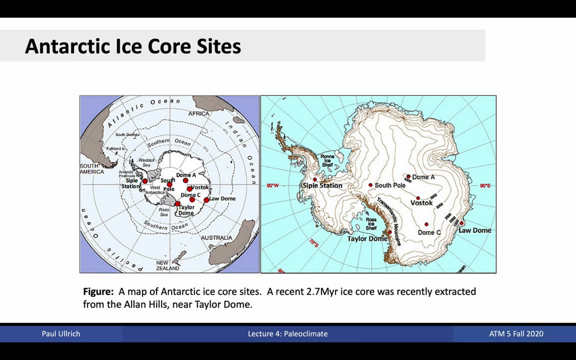 New Zealand, Indonesia, Greenland and Antarctica. The longest ice core records have actually been pulled from Antarctica, which has been frozen for the past 12 million years. However, reaching back that far is pretty difficult, because it's rare to come across such cleanly layered ice cores. The Vostok ice core is perhaps the most recognizable by name. 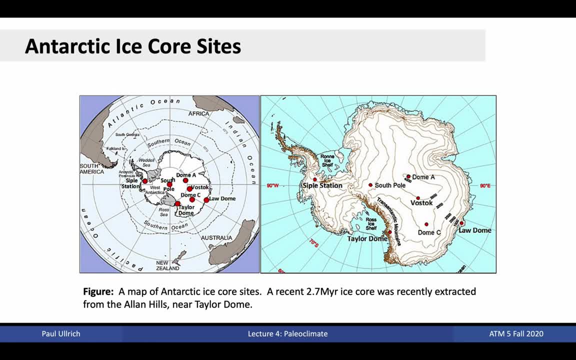 and gave us a usable record of ice to 3,310 meters depth after drilling between 1990 and 2007.. This ice core has enabled us to look 420,000 years into the past. In 2006,, a European group, 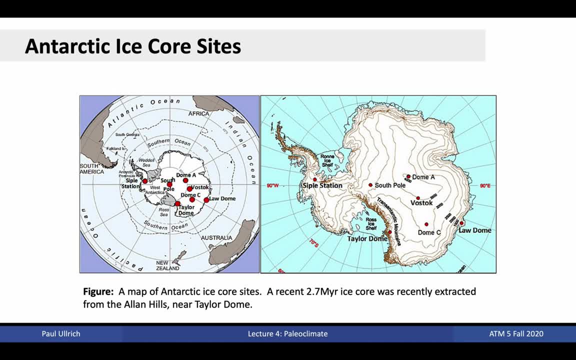 known as EPICA, extracted an ice core from Doha, Africa and Africa. The ice core was a dome sea in Antarctica reaching 3,260 meters in depth before hitting bedrock. Usable data from this drilling project provided us with a usable record up to 800,000 years ago. In 2016,, cores 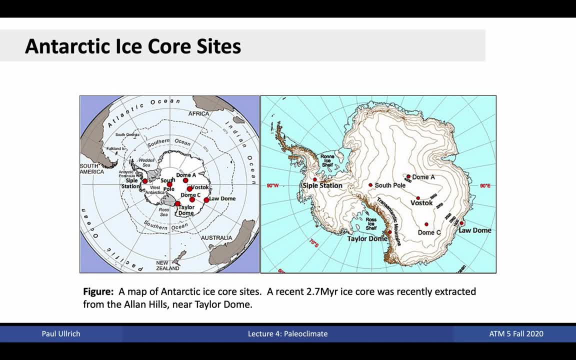 were retrieved from the Allen Hills. Using radiometric dating, they found that it included ice up to 2.7 million years ago. This ice core remains under analysis. Ice cores also are commonly pulled from the Alps, Alaska and Antarctica. The ice cores are also. 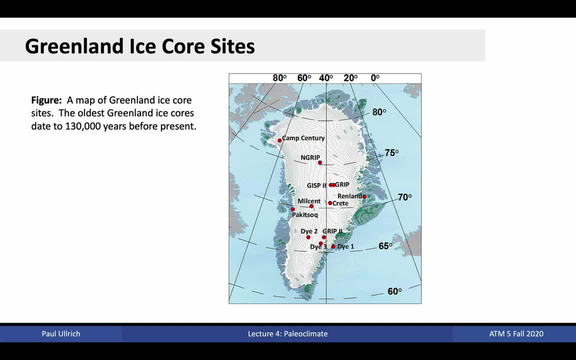 pulled from Greenland. In 2010,, a 2,537-meter core was drilled in Greenland, providing a climatic record to 128,500 years ago, with more of a focus on the northern hemisphere. Greenland's relative accessibility compared with Antarctica have also made it a popular destination for students working. 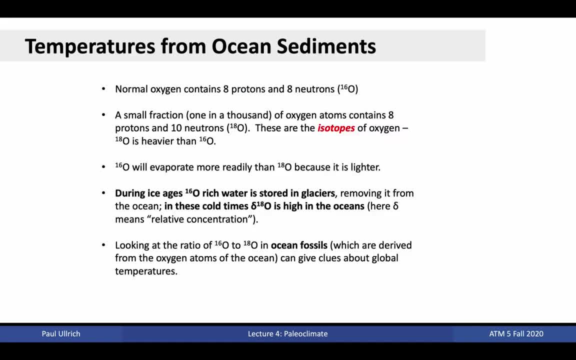 on projects in paleoclimate and the cryosphere. Of all the proxies available to us, our longest record of temperatures have come from the slow accumulation of ice in the Alps, Alaska and Antarctica. By looking at isotope ratios of oxygen we can actually build a reasonably accurate. 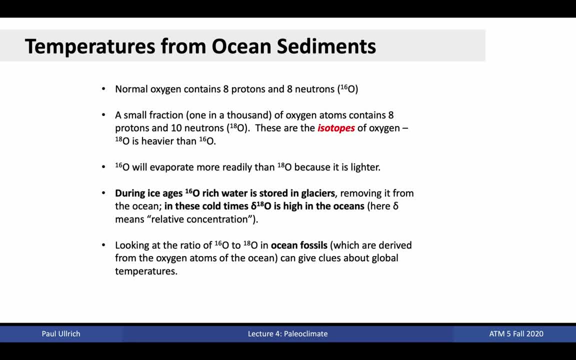 record of past temperatures. The basic procedure is a bit technical, but it's worthwhile to understand as a smart solution pursued by scientists. So oxygen is a common ingredient in life and also present in water. However, oxygen comes in a few different forms depending on the number of neutrons in the atom, known as isotopes, The most abundant. 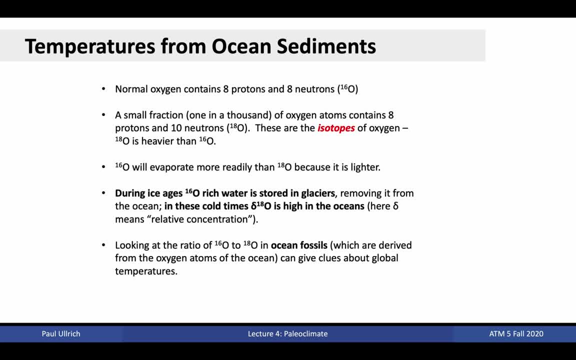 form of oxygen is the oxygen of the atmosphere. The oxygen of the atmosphere is the oxygen of the atmosphere. The oxygen of the atmosphere is the oxygen of the atmosphere. The oxygen of the atmosphere consists of eight protons and eight neutrons and is known as 16O because it weighs 8 plus 8.. 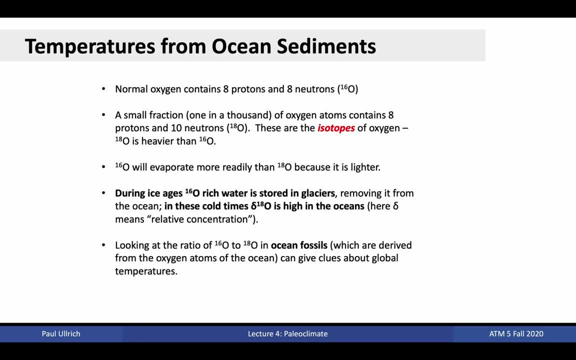 However, there's another stable form of oxygen that contains eight protons and 10 neutrons, known as 18O. Because it has more neutrons, this latter form of oxygen is a bit heavier than the former. Because 16O is slightly lighter than 18O, it requires a bit less energy to evaporate from. 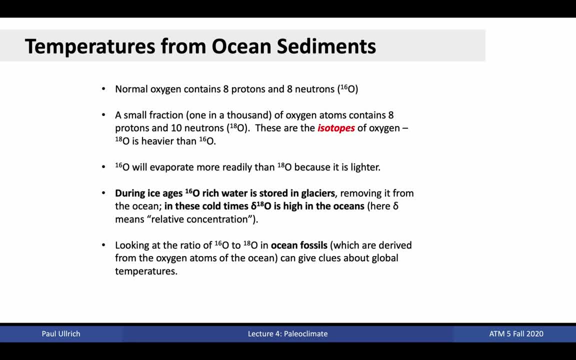 ocean water and so atmospheric water vapor has a higher ratio of 16O. So if we look at the 16O to 18O than ocean water. During cold periods, this 16O water will be trapped in the form of land. 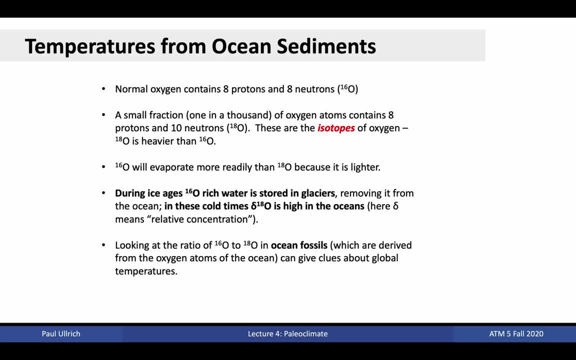 ice, and so won't be used to replenish ocean water. In these cold times, the relative concentration of 18O and 16O will be higher than in ocean water. Similarly, during warm periods, land ice will melt and replenish 16O in ocean water, driving up the 16O concentration in oceans Around 542. 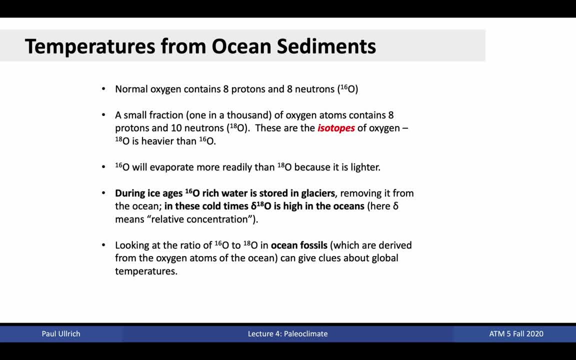 million years ago, the ocean water was the highest concentration of 16O in the world, So life arose in the oceans that used the oxygen in ocean water to build calcium carbonate shells. When these organisms died off, they fell to the ocean floor, where they accumulated over time in 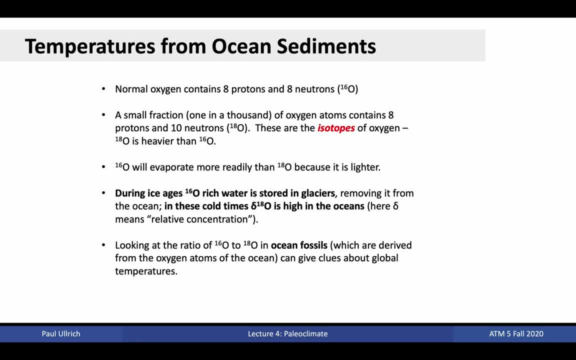 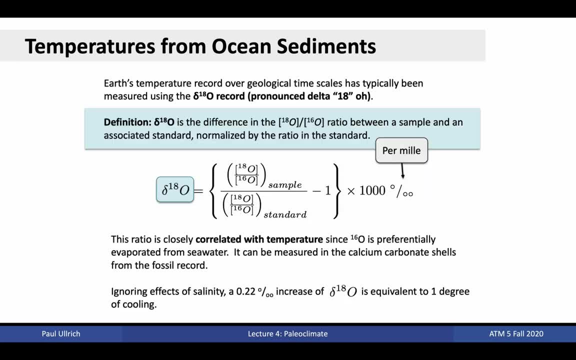 the form of ocean sediments. By combining radiometric dating with an analysis of the relative abundance of 18O, we can gain an understanding of the temperatures of that time. The relevant measure of 18O and 16O concentration in the world's oceans is determined by a quantity. 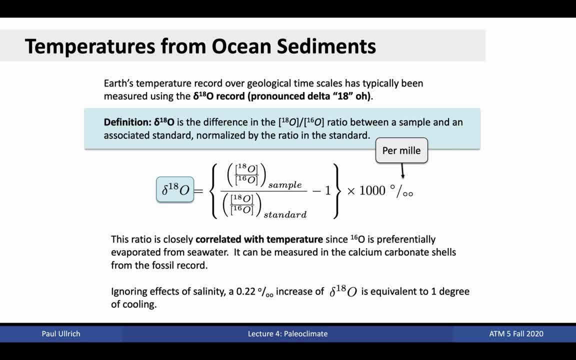 known as delta 18O. By definition, delta 18O is the difference in the 18O divided by 16O ratio between a sample and an associated standard normalized by the ratio in that standard. As mentioned, this ratio is closely correlated to temperatures generally, a 0.22 per mil increase in delta 18O. 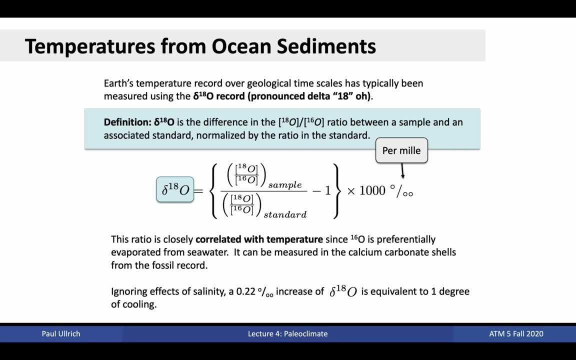 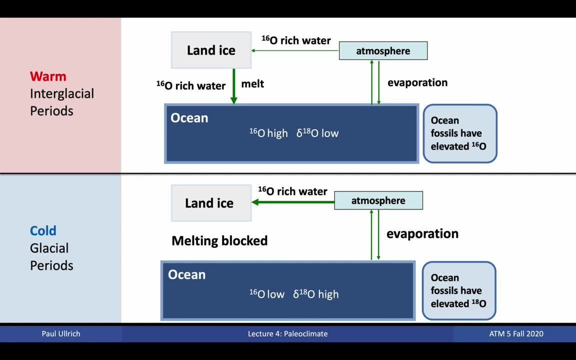 that is, more 18O in seawater. This is equivalent to 1 degree of cooling. This figure provides a graphical depiction of why delta 18O is low in the oceans during warm interglacial periods and high during cold glacial periods. During warm periods, 16O naturally moves. 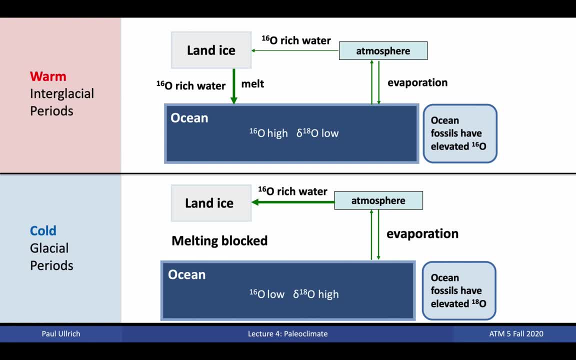 through the hydrologic cycle, evaporating from the ocean, precipitating out over land, potentially forming land ice that then melts back into the ocean. During cold periods, after 16O precipitates out over land, melting is blocked because the low temperatures keep it locked up in ice. Consequently, 16O is depleted in the oceans. 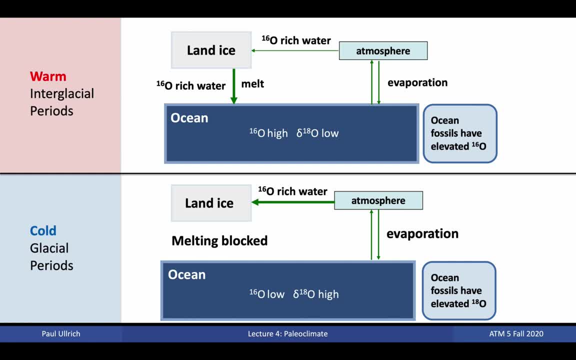 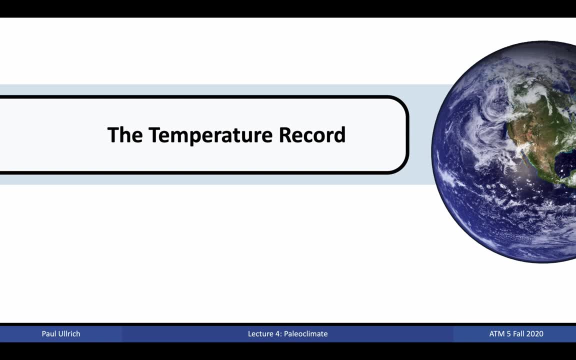 and the value of delta 18O becomes high. The relative concentrations of these two isotopes is then reflected in ocean fossils. Now that we've understood how scientists have used proxies to measure historical temperatures, let's look at our most up-to-date understanding of how the temperature record has changed. 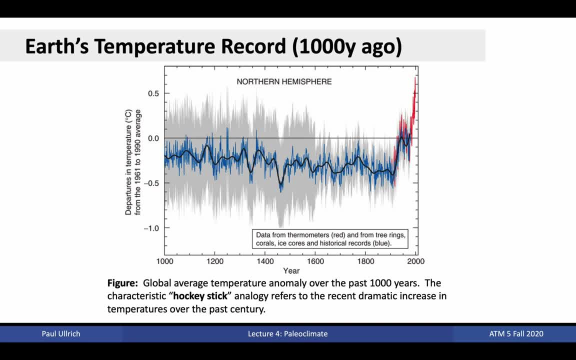 Data from thermometers, tree rings, corals, ice cores and historical records are combined in this plot to give us a rough timeline of temperatures over the past thousand years relative to the 1961 to 1990 average Prior to 1900, it's our understanding. 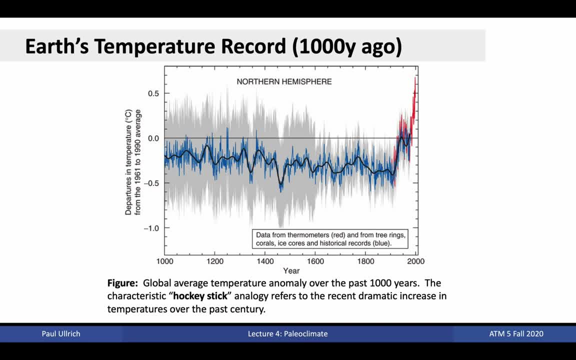 that global temperatures were cooling slightly, although there was significant year-to-year variability. A period known as the medieval warm period, extended from 950 AD to 1250 AD. although this warmth was mainly confined to the northern hemisphere, This was followed by the little ice. 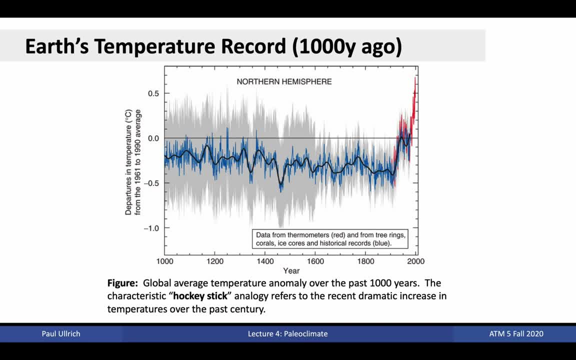 age, which extended from 1350 AD to 1250 AD. This was followed by the little ice age, which extended from 1300 AD to 1860 AD. During this period, mountain glaciers expanded in many regions of the world. This particular temperature time series has also been known collectively as the hockey stick. 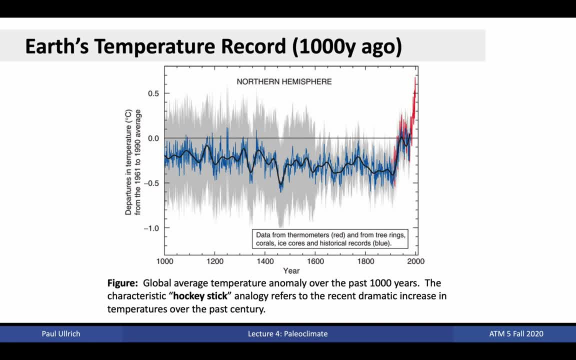 diagram in the context of climate change. This is because the relatively stable climate record, followed by an acceleration in temperatures from the 1930s through 2000,, looks vaguely like a hockey stick turned on its side. As discussed last time, the temperature rise between the pre-industrial 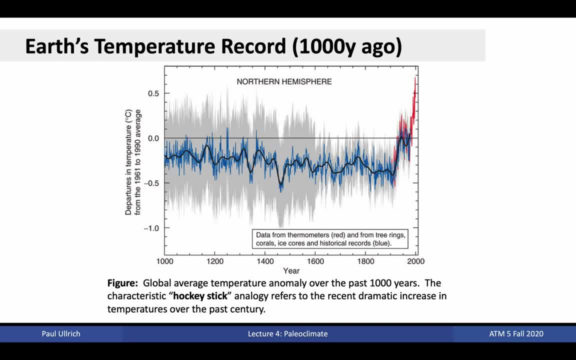 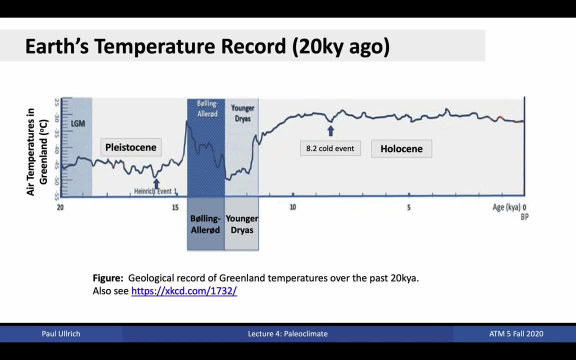 period and the present is. the temperature rise between the pre-industrial period and the present is around 1°C. Using the geological records from Greenland, we are able to extend the temperature record back over the past 20,000 years. This allows us to clearly see the relative stability. 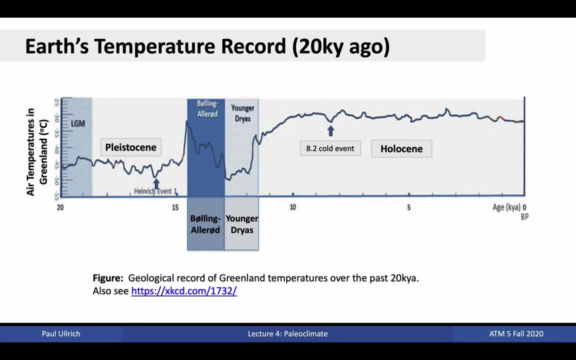 of temperatures in the Holocene, a period in the Earth's history over the past 11,000 years where we have witnessed the rise of human civilization. There is no doubt that human civilization has benefited from the relatively stable climate of this period. 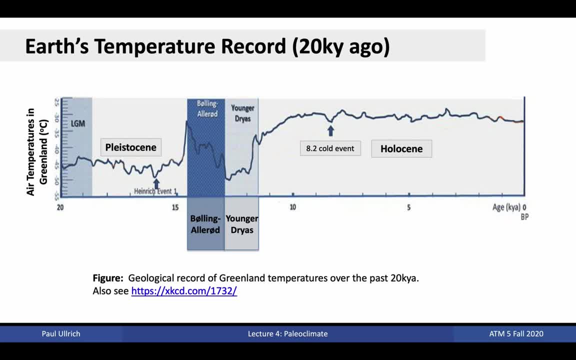 Before the Holocene came the Pleistocene, a period lasting from 2.6 million years before present to 11,700 years ago. This period was characterized by repeated glacial and interglacial cycles. During these glacial periods, up to 30% of the Earth's surface was covered in ice. 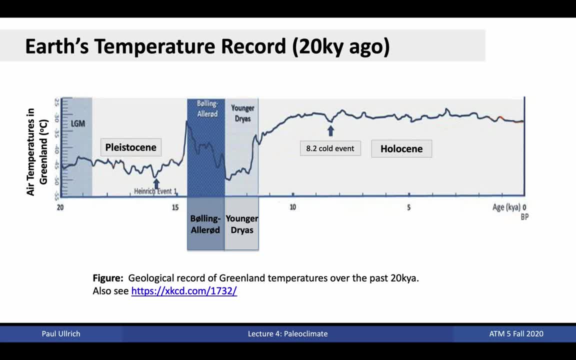 The fauna of the Pleistocene was essentially the same as modern day, but with many more large land mammals such as mammoths. Modern humans evolved and spread out over the planet during this period, and the cold temperatures drove lower sea levels and created natural land bridges between continents. 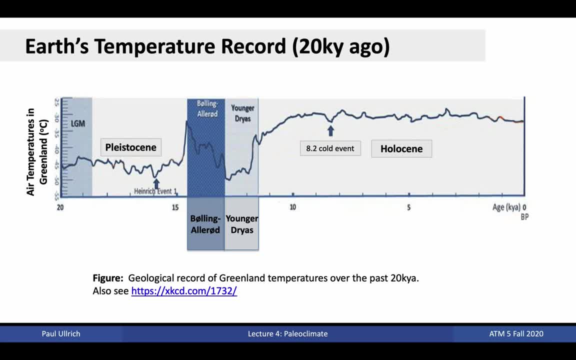 Between the Pleistocene and the Holocene there was a period of climatic upheaval. The first change was a sudden warming known as the Bolling-Allerod, which was characterized by an abrupt warming and transition to interglacial. This sudden warming led to rapid melt of overland. 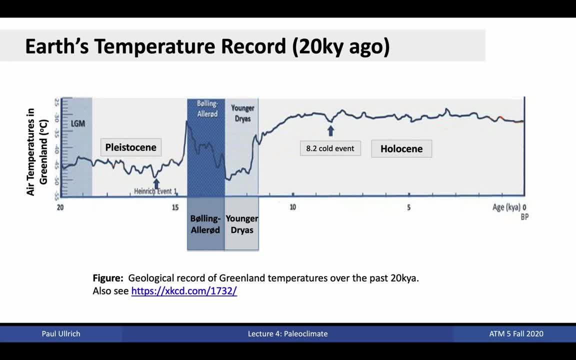 glaciers and produced a meltwater pulse that triggered sea-level rise of 16 meters. This sudden dump of fresh water into the This sudden dump of fresh water into the North Atlantic blocked the transport of warmer equatorial waters into this region and drove reglaciation and colder temperatures in a period known as the Younger Dryas. The Younger Dryas. 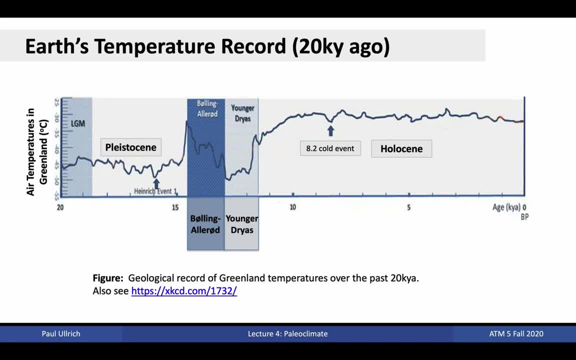 persisted for about 1.5 thousand years before the advent of the Holocene. To learn more about the climate of this period, you can check out the xkcd comic actually linked here. It does an excellent job of emphasizing how these natural changes in temperature occur gradually over long periods. unlike the warming we've experienced in the past. This is an example of how natural changes in temperature occur gradually over long periods, unlike the warming we've experienced in the past. This is an example of how natural changes in temperature occur gradually over long periods, unlike the warming we've experienced in the past. 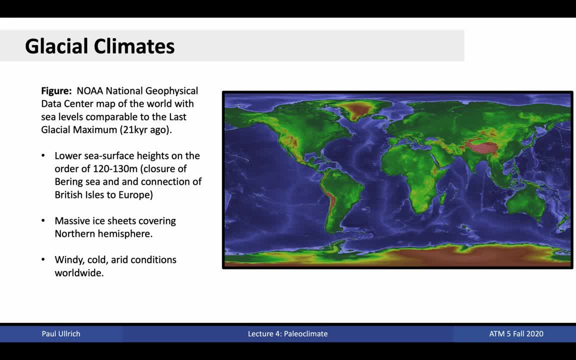 Under a cold glacial climate, the Earth looked more like the maps shown here, With cold ocean waters trapped in land ice. the sea surface was 120 to 130 meters lower than today, or around 400 feet. This led to the closure of the Bering Strait. 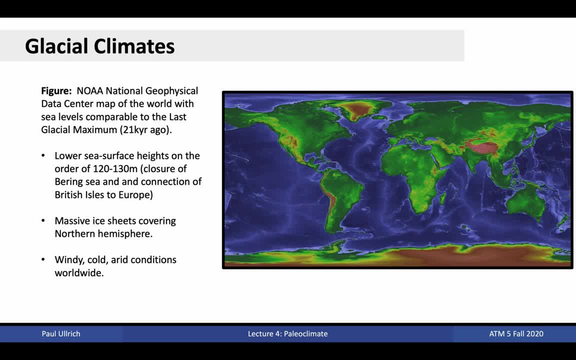 which connects Asia and North America, as well as connecting the British Isles to Europe. Presumably, it would have been harder to argue for Brexit under these circumstances. Nonetheless, massive ice sheets covered much of the Northern Hemisphere. Cooler air temperatures also meant less water in the atmosphere, so conditions worldwide were windy, cold and dry. 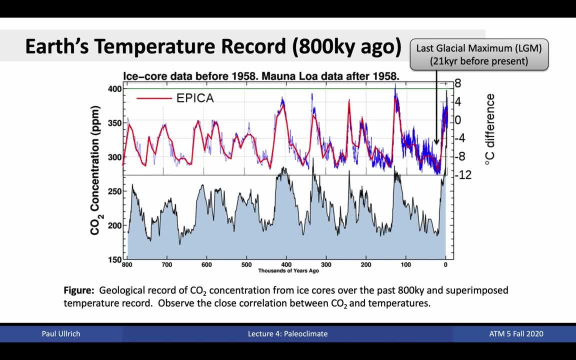 With ice core data from Antarctic ice cores, primarily the Dome Sea ice core, we can extend the temperature record to 800,000 years before present. Here we see clearly that the Pleistocene is characterized by roughly 100,000 year shifts between glacial and interglacial periods. 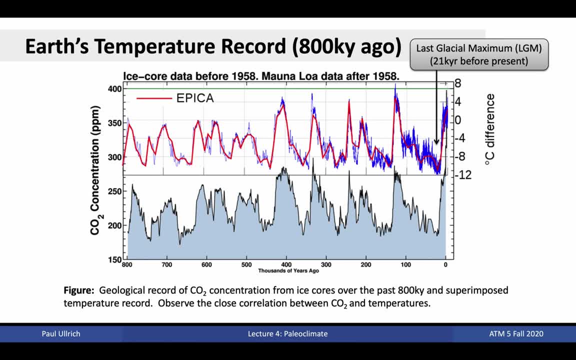 between glacial and interglacial periods, with the larger ice sheets covering much of the northern hemisphere, The last glacial maximum, abbreviated as LGM, occurring about 21,000 years ago. Temperature swings between these periods are on the order of 10 degrees Celsius. 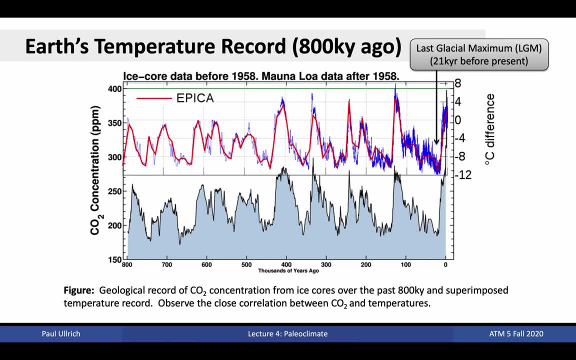 Atmospheric carbon dioxide concentrations obtained from air bubbles in the ice core are shown in the lower plot here and correspond well with the observed temperature record. This is indicative of the intimate connection between carbon dioxide and global temperatures. Colder periods are characterized by CO2 levels around 100,000.. 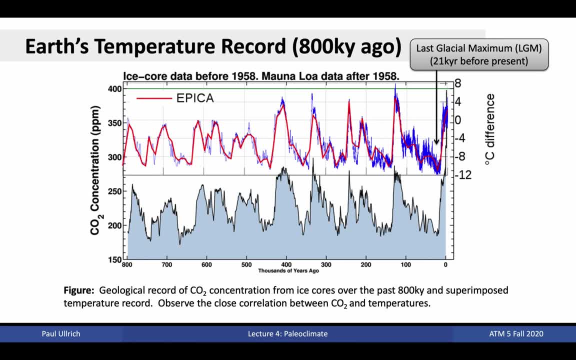 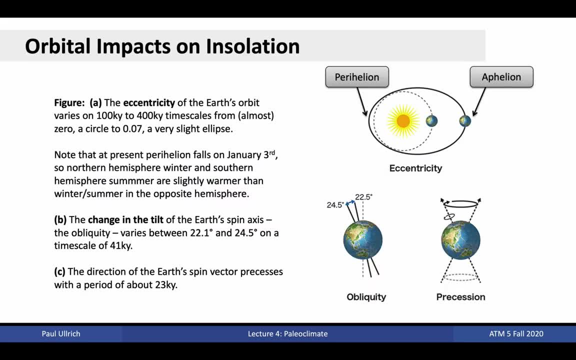 Colder periods are characterized by CO2 levels around 180 parts per million, whereas warmer periods are characterized by CO2 levels more around 280 parts per million. So why is there a 100,000 year oscillation in glacial and interglacial periods? 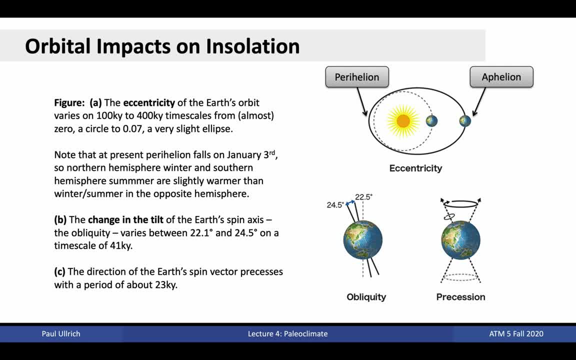 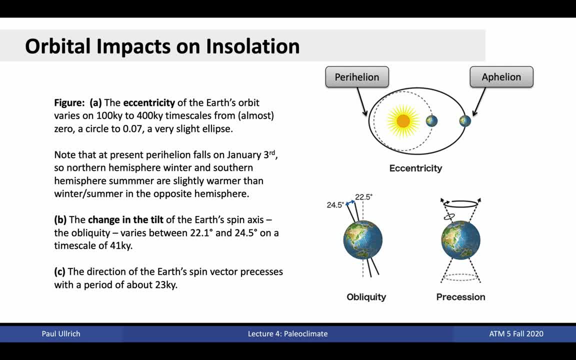 Over time, this value changes from almost zero, which describes a completely circular orbit, to about 0.07, which is a very slight ellipse. A more elliptical orbit is characterized by more severe seasonal shifts in temperatures. At present, perihelion, or the point where the Earth is closest to the sun, 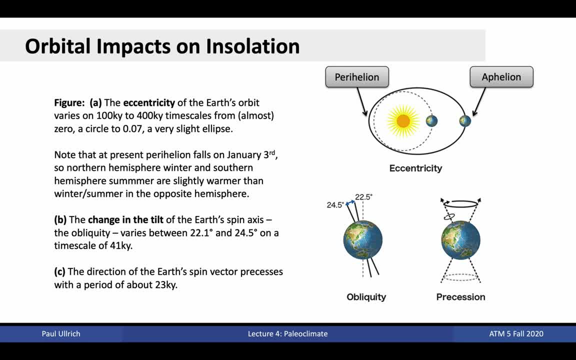 falls on January 3rd, meaning that the northern hemisphere winter and southern hemisphere summer are slightly warmer than winter and summer in the opposite hemisphere. Obliquity refers to changes in the tilt of the Earth. At present, the Earth is tilted at 23.5 degrees. 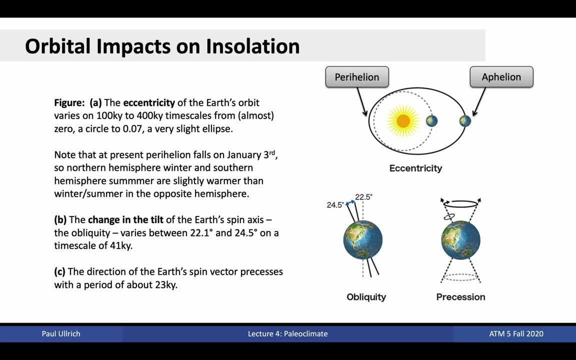 but the Earth wobbles slightly over long time periods, like a gyroscope, with the tilt moving between 22.1 degrees and 24.5 degrees on a time scale of approximately 41,000 years. The final orbital variable precession. 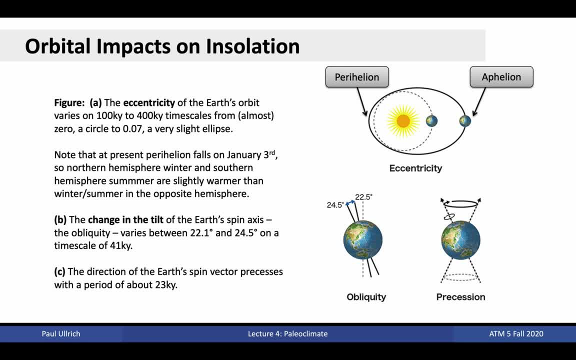 refers to the direction of the Earth's axis. This changes over a period of roughly every 23,000 years. This means that approximately 11,500 years ago, the tilt was the opposite of what it was today, Namely December was the peak of summer in the northern hemisphere. 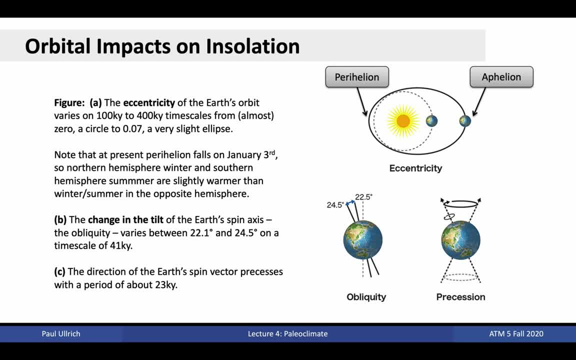 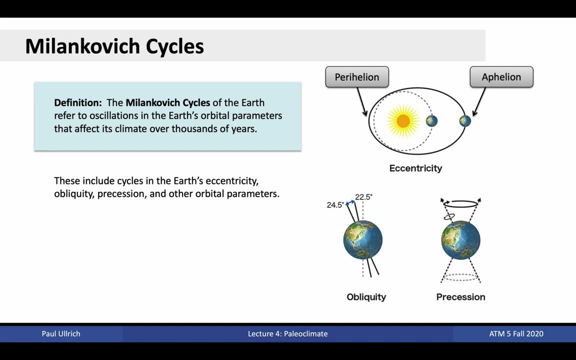 At present, our north pole axis points towards the star Polaris, but 2,000 years ago the pole star referred to its neighbor Kochab, which is part of the Little Dipper. The combination of these three orbital variables gives rise to what is known as Milankovitch cycles. 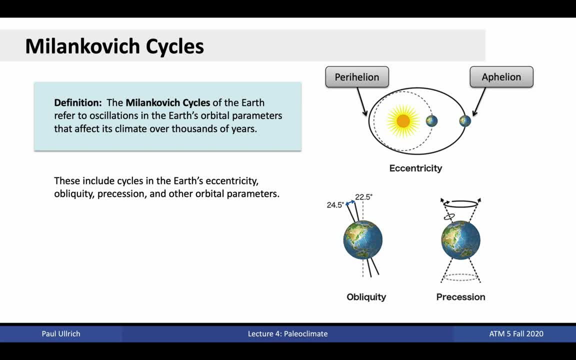 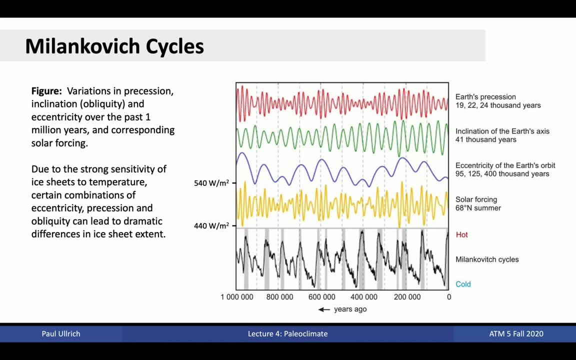 oscillations of the Earth's orbital parameters that affect its climate over thousands of years. Milankovitch cycles have a significant effect on solar forcing in the subpolar regions, where the amount of energy received can vary between 440 watts per square meter. 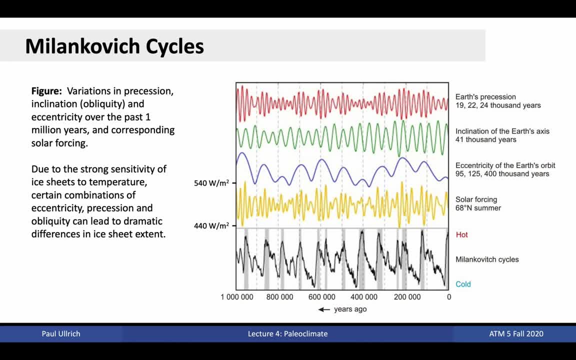 and 540 watts per square meter, or about 25%, depending on where the Earth is in its cycle. Due to the strong sensitivity of the ice sheet extent to variations in temperature, the Milankovitch cycles can lead to dramatic differences in ice sheet extent. 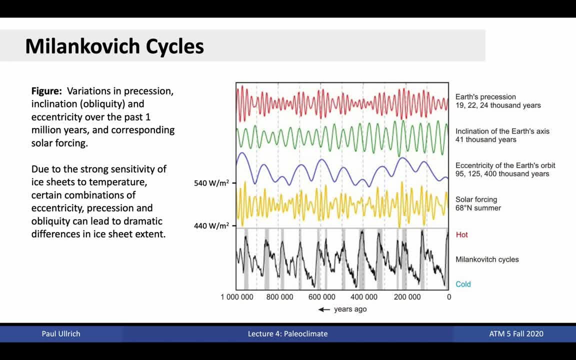 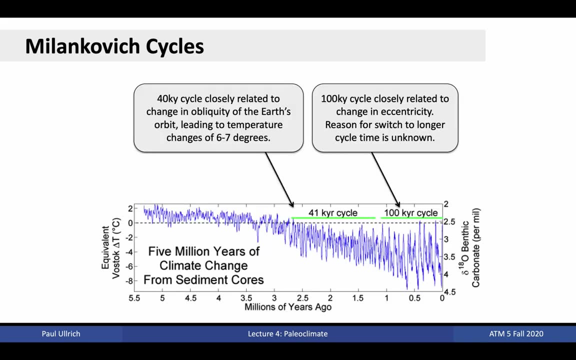 That is, under relatively low radiative conditions, we would expect the ice sheet to grow, Whereas under the 540 watts per meter squared conditions we would expect the ice sheet to be in retreat. Looking over the entire temperature history of the Pleistocene. 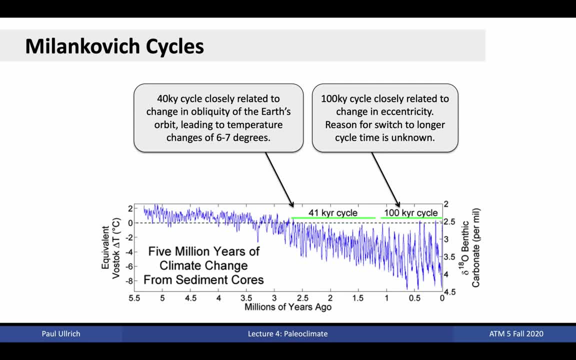 we see two recent periods of glacial slash interglacial oscillations. At present, the 100,000-year eccentricity contribution dominates the climate signal and drives shifts between glacial and interglacial cycles. However, one million years before present to the beginning of the Pleistocene, the climate was characterized by a 41,000-year. 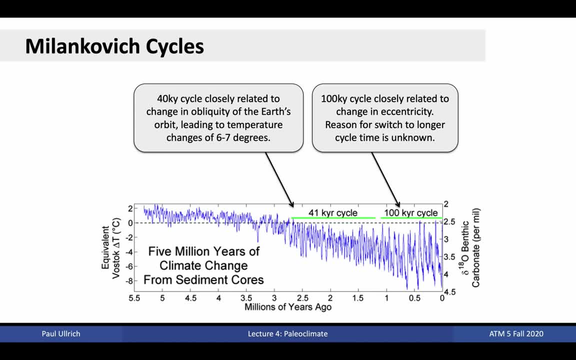 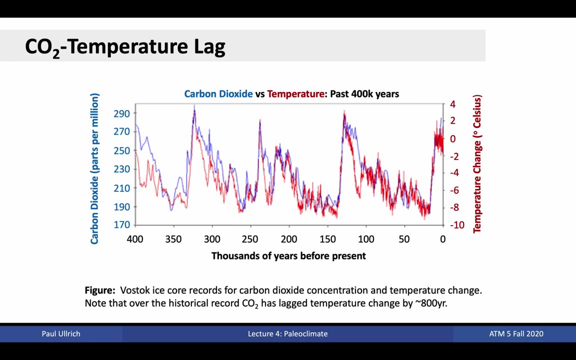 cycle more closely associated with changes in obliquity of the Earth's orbit. The reason for this shift remains unknown and an area of active research. The climate of the past 400,000 years revealed by the Vostok Ice Core also provides evidence of a lag between carbon dioxide. 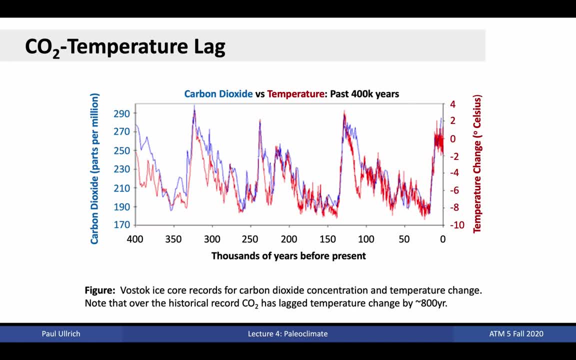 concentration and global temperatures. Historically, we have seen carbon dioxide concentrations peak around 800 years after the corresponding peak in temperatures. Some in the climate change denier community have latched onto this to argue against the relationship between carbon dioxide and temperature. After all, if CO2 lags temperatures, then it couldn't have been the factor driving the rise. 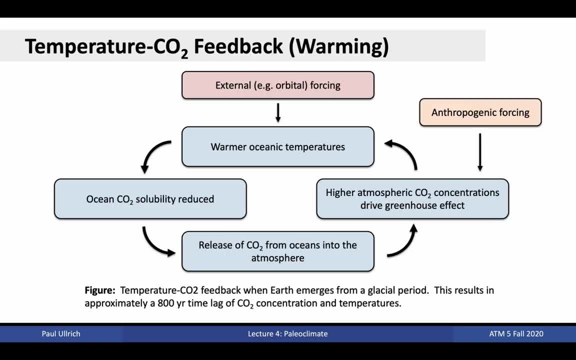 in historical temperatures. However, the explanation is actually a fairly simple consequence of the connection between CO2 and temperature. You might notice that when you warm up soda it tends to taste flat. This is because warmer water or soda is not as good at holding onto carbon dioxide. 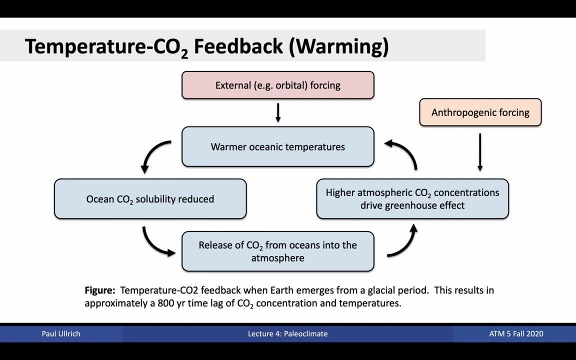 Namely when it warms up, it releases that CO2 into the air. The ocean behaves in the same way: As orbital changes drive up ocean temperatures, the solubility of CO2 in ocean water is reduced and CO2 is released into the atmosphere, Because CO2 then induces further. 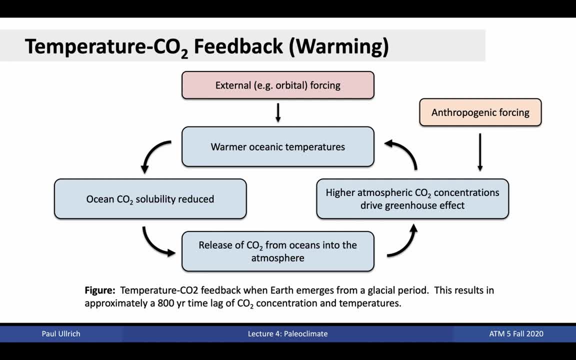 warming. this drives up the greenhouse effect, which in turn drives warmer ocean temperatures. The lag between the warmer temperatures and CO2 increases on the order of 800 years. This feedback cycle is then responsible for rapidly driving the Earth out of a glacial period and into the ocean. 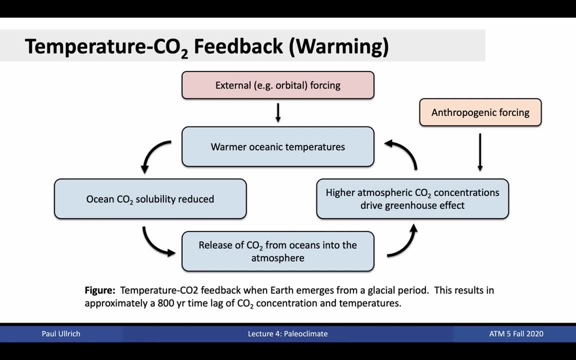 The human influence on this cycle is over. here on the right. Instead of modifying ocean temperatures directly, we are instead adding more CO2 to the system, which then has the consequence of warming ocean temperatures and driving more CO2 release. So in this case, we expect CO2 increase to lead. 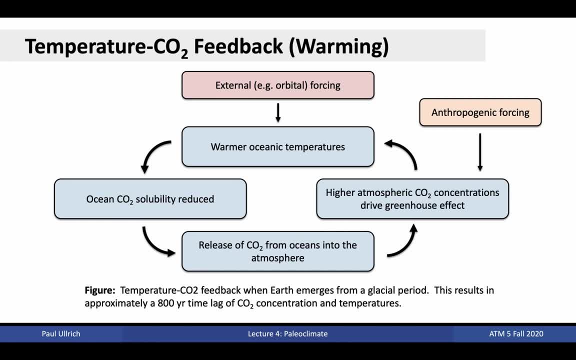 to ocean temperatures to increase. Consequently, once those ocean temperatures increase, the solubility of CO2 in the oceans will decrease. This will result in more CO2 being released to the atmosphere, and thus it will provide a driver for this feedback cycle, driving up temperatures even farther. 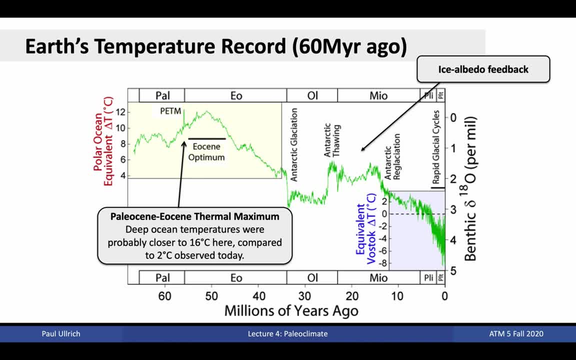 We can now turn our attention back to the Earth's temperature record. Using ocean sediments, we can look even farther back over the past 60 million years. What becomes clear is that temperatures have generally been much higher in the past, up to 12 degrees Celsius warmer than present. Before the Pleistocene, there was a period of 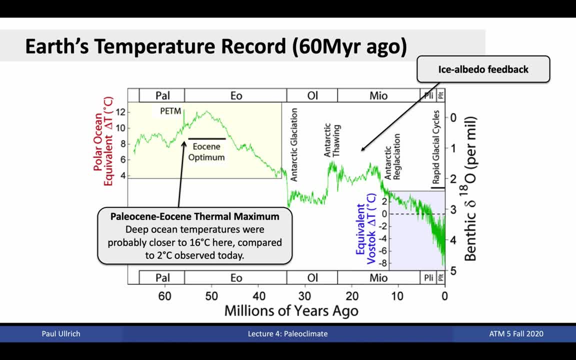 cooling that included more CO2 than present. This is because the temperature of the ocean reclassification of the Antarctic approximately 12 million years ago, Feedbacks between surface ice and temperatures drove down global temperatures during reclassification and temperatures have been descending ever since The Antarctic was ice-free between approximately 25 million years. 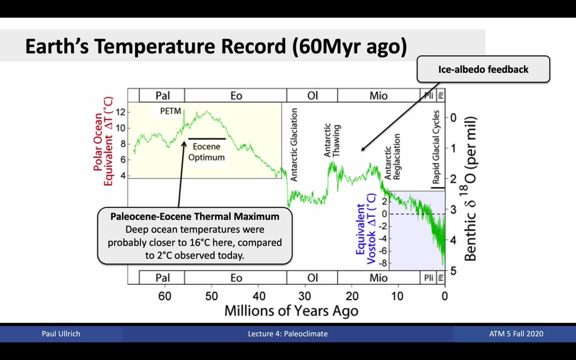 ago and 12 million years ago, a period that is associated with higher temperatures, But it was again glaciated between 34 and 25 million years ago. Before this period was the Eocene and Paleocene: two-time periods of cooling that included more CO2 release. This is because the temperature of the Antarctic was higher than the temperature of the Eocene Before. this period was the Eocene two-time periods of cooling that included more CO2 release. This is because the temperature of the Antarctic was higher than the temperature of the Eocene Before. this period was the Eocene. 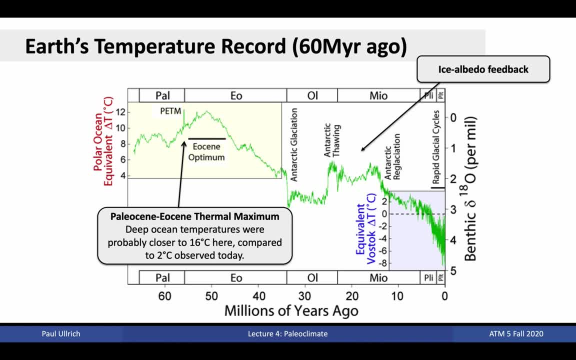 The period of warmest temperatures is known as the Eocene Optimum. At the boundary of the Paleocene and Eocene, a dramatic spike in temperatures occurred, known as the Paleocene-Eocene Thermal Maximum, or the PETM. This event was associated with deep ocean temperatures likely. 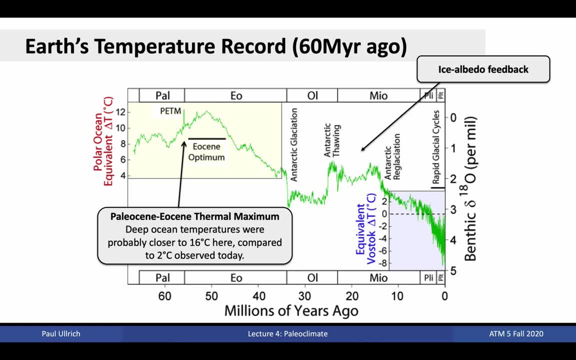 closer to 16 degrees Celsius, compared with the 2 degrees Celsius today. Palm trees and cold-blooded reptiles were found at the North Pole. during this time, The temperature of the Eocene was higher than the temperature of the Paleocene. This period is often studied as a proxy for what 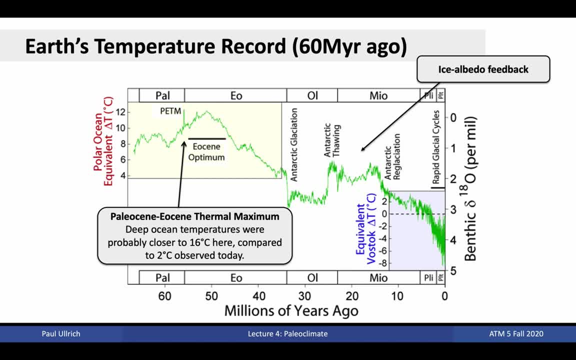 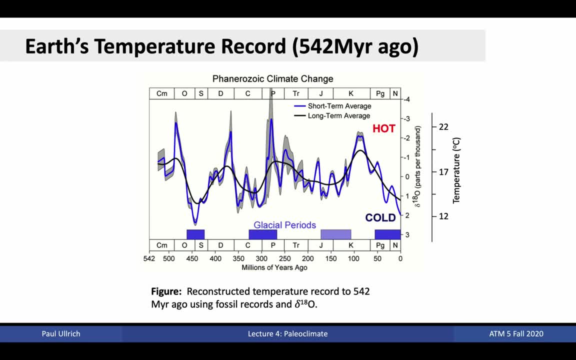 we can expect under anthropogenic or sudden climate change. Looking back to the emergence of these sediment records nearly 542 million years ago, we see that the Earth has oscillated between extended warm and cold periods on timescales of tens of millions of years. Here, glacial periods, including today, refers to times when 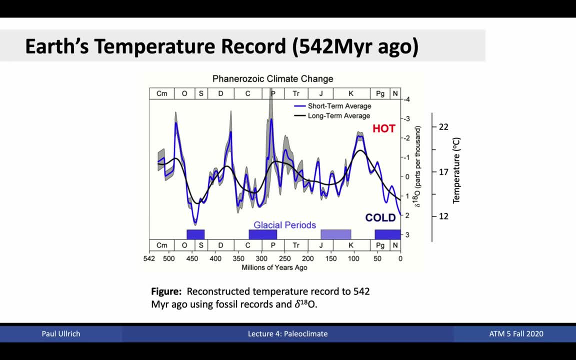 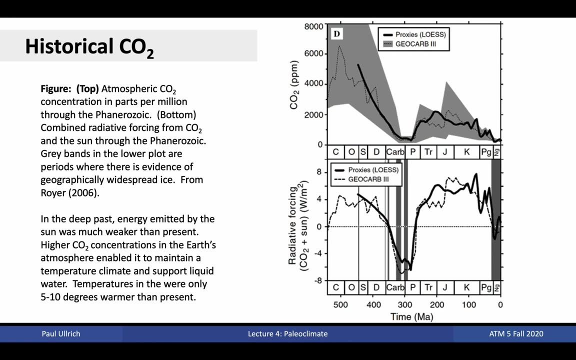 there is evidence that ice persisted over the surface of the planet. At the current rate of warming, it is anticipated that the current glacial period will end in the next 500 years. Historical carbon dioxide levels can be estimated using available proxies. What is generally? 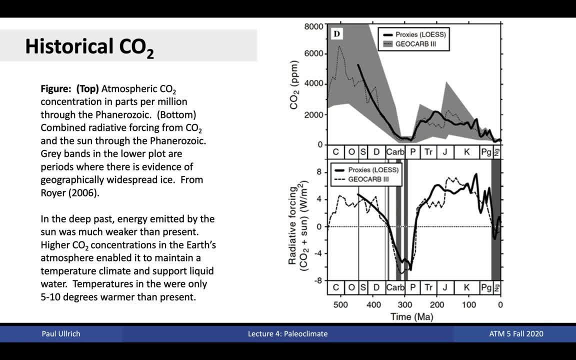 known is that during warm periods, CO2 levels are elevated and during cold periods, CO2 levels are in decline. During the reign of the dinosaurs, from the Triassic 230 million years ago through the Cretaceous 66 million years ago, carbon dioxide levels were around. 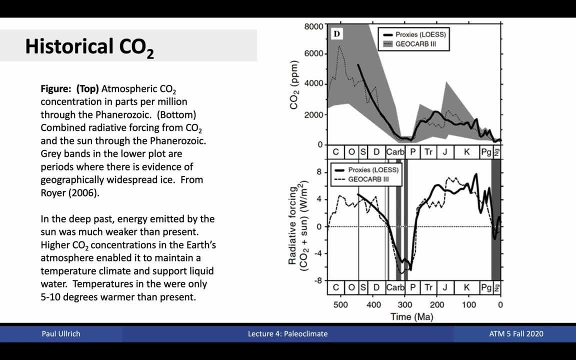 2,000 parts per million, or about four times today's levels. Before that, there was a period of relatively low CO2 after millions of years of CO2 decline. During the emergence of life on Earth, CO2 levels were likely around 4,000 parts per million, although uncertainty here is large in 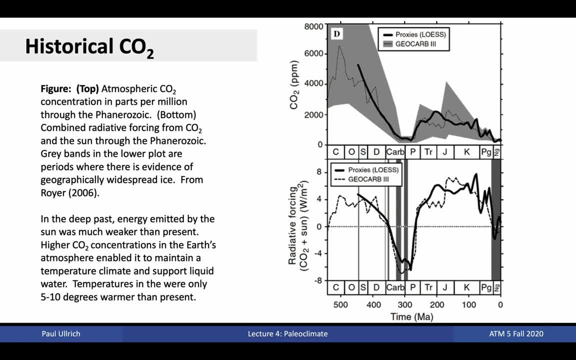 these measurements. For millions of years, the first life breathed in this carbon dioxide and breathed out oxygen, building up the oxygen atmosphere of today. So why weren't temperatures much higher then than today? Well, we know that over timescales of hundreds of millions of years, solar output has been steadily increasing. The Earth of 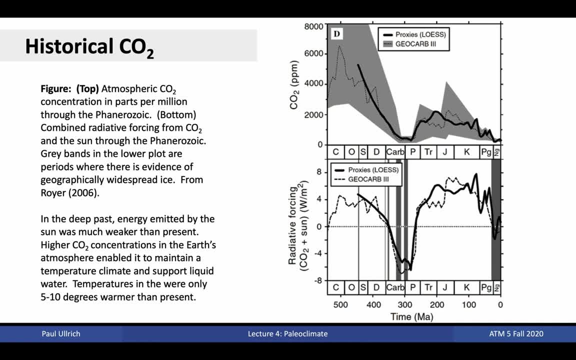 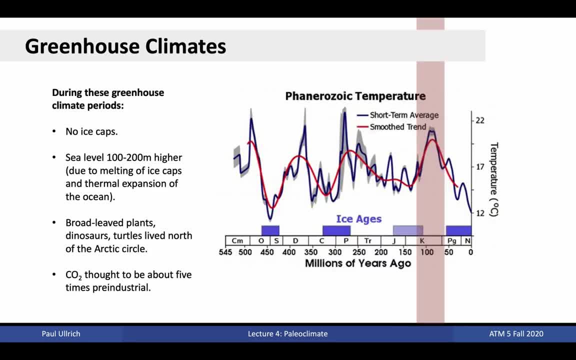 planet's energy. CO2 was depleted to around 30% of the planet's energy. CO2 was depleted to around 30% of the planet's energy. CO2 was depleted to around 30% of the planet's energy. Let's now take a look at what the earth looked like under the greenhouse climates of the past. 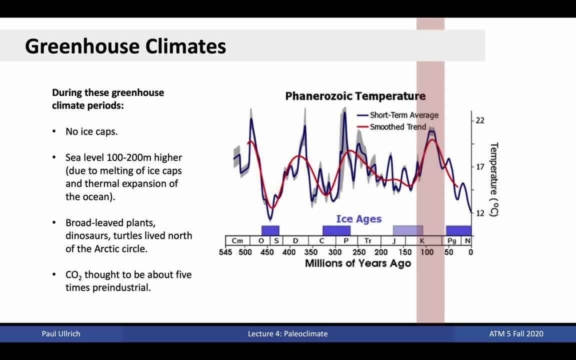 If anthropogenic climate change continues at the current rate, this is where we see the world heading. During the Cretaceous period, 100 million years ago, the world was about 10 degrees Celsius warmer than present day. During this time, there were no ice caps, Melt of land, ice and thermal 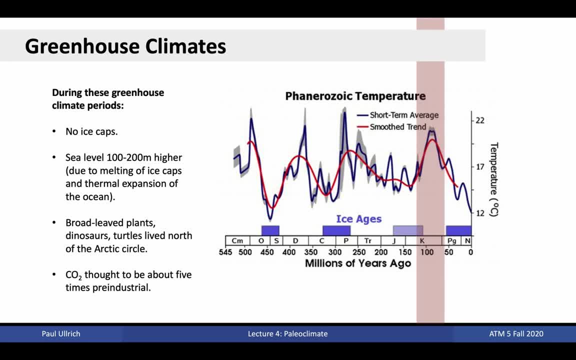 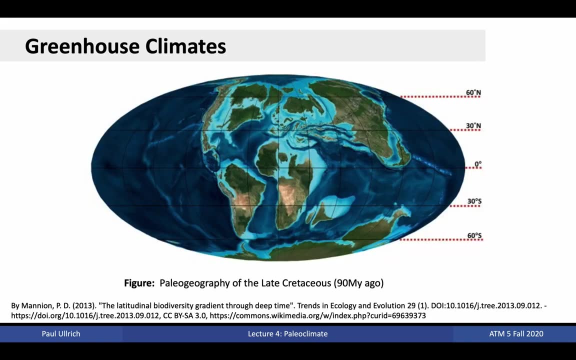 expansion of ocean water meant that sea levels were 100 to 200 meters higher, or 300 to 600 feet. We know that from this period, broad-leaved plants such as palm trees, dinosaurs and turtles lived north of the Arctic Circle in the warm waters around the North Pole. Here's a likely 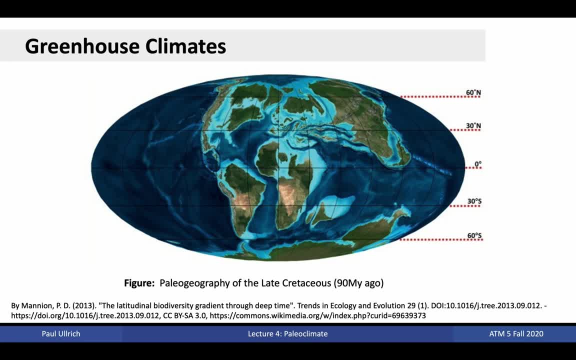 picture of what the world looked like 90 million years ago during this greenhouse period. At the time, the continents were far more clustered and shallow seas covered much of the planet. North America at the time had a massive inland sea responsible for marine fossils being spread. 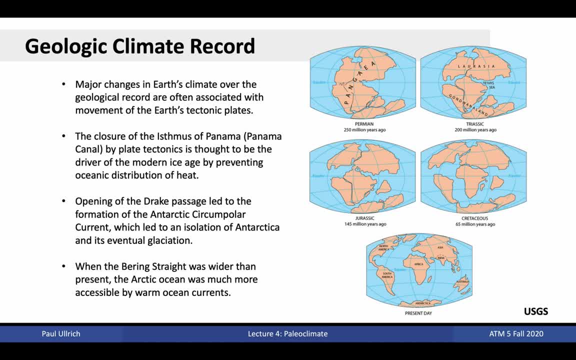 from Colorado to Nevada. The geologic record of the planet can give us some clues for some of the major drivers of the earth's climate. Some of these changes in climate were associated with how the continents allowed water to circulate around the earth system When the isthmus of Panama closed, where the Panama 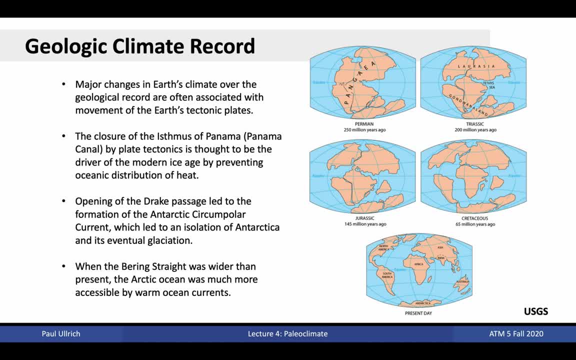 Canal is now located. warmer equatorial Pacific waters could no longer circulate into the Atlantic. This is hypothesized to be a major driver of the modern ice age. When the Drake Passage opened between South America and Antarctica, the Atlantic waters could circulate freely around Antarctica. This set up the Antarctic. 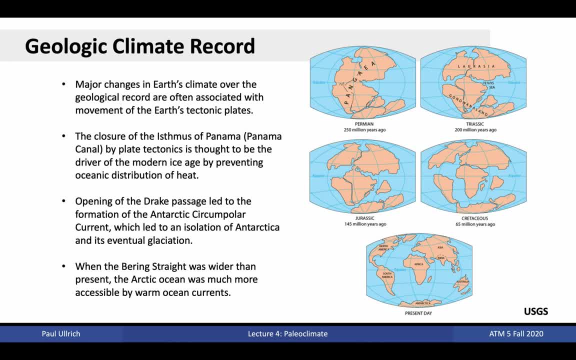 Circumpolar Current, a region of fast-moving waters around Antarctica. This isolated the continent and led to its eventual glaciation or its covering with ice. When the Bering Strait between North America and Asia was wider than present, the Arctic Ocean was also far more. 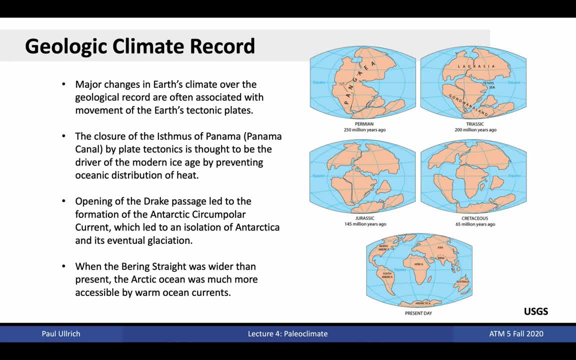 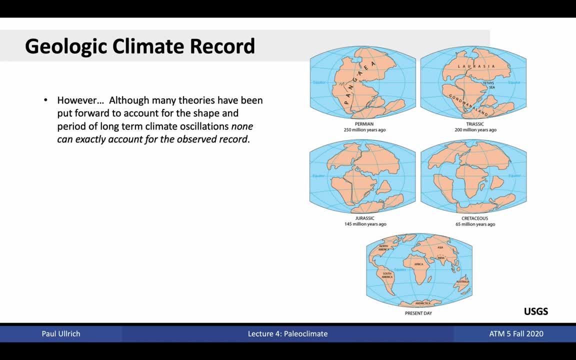 accessible by warm ocean currents, which suppressed sea ice and made this ocean far more inhabitable. Nonetheless, regardless of these observations, work on understanding Earth's climate history continues. At present, there is no comprehensive theory that fully accounts for the observed climate record of the past.